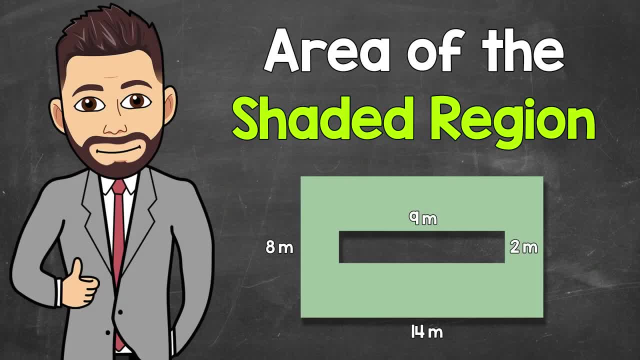 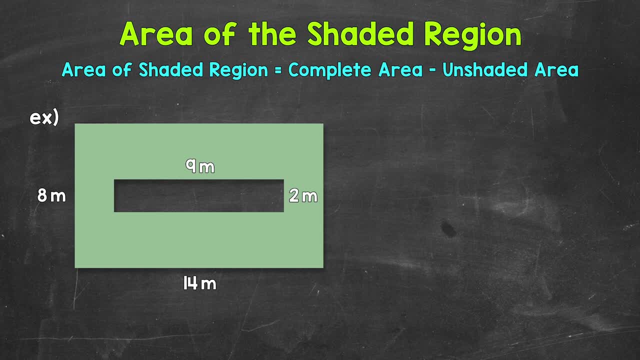 Welcome to Math with Mr J. In this video I'm going to cover how to find the area of the shaded region And, for our example, we have a rectangle inside of a rectangle, So basically a rectangular hole in the middle of the larger rectangle. 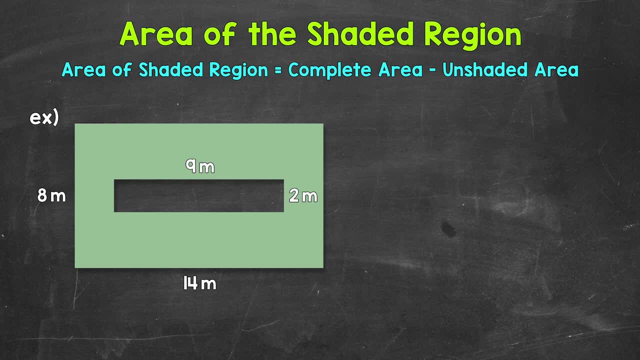 We need to find the area of the shaded region. so the green, We do this by finding the area of the larger outside rectangle and subtracting the area of the smaller inside rectangle. Let's start by finding the area of the larger outside rectangle. 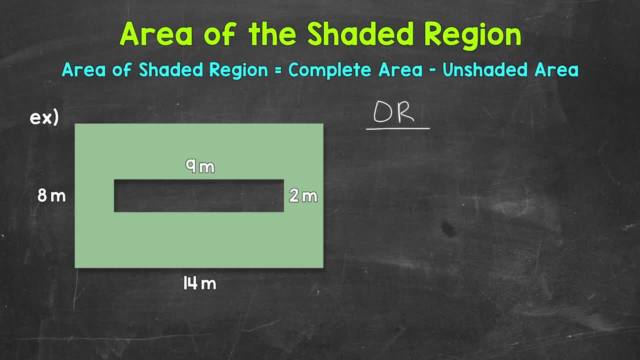 So I'm going to put OR for outside rectangle. So we are finding the complete area of that larger outside rectangle. Area equals and we will use length times width in order to find the area. So now we need to plug in the length and the width. 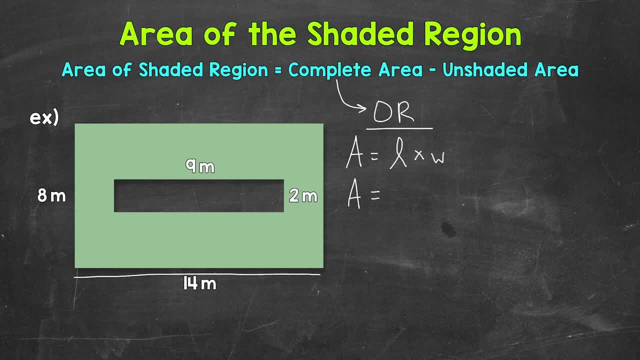 So area equals. I'm going to use 14 for the length and 8 for the width, So 14 times 8.. 14 times 8, that's going to give us an area of 112, square meters And that's the complete area of that larger outside rectangle. 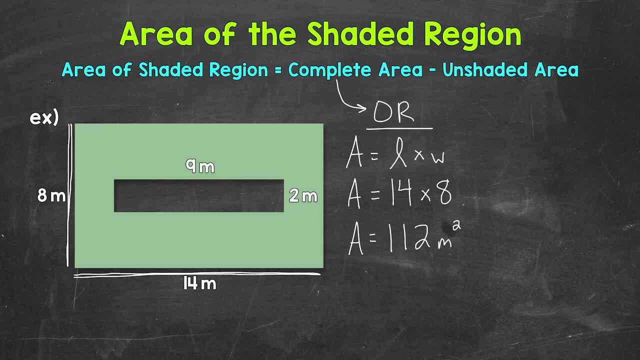 Now we need to subtract the area of the smaller rectangle, We need to take out the rectangular hole, so to speak, And that's going to give us the area of the shaded region. So let's now find the area of the inside rectangle. 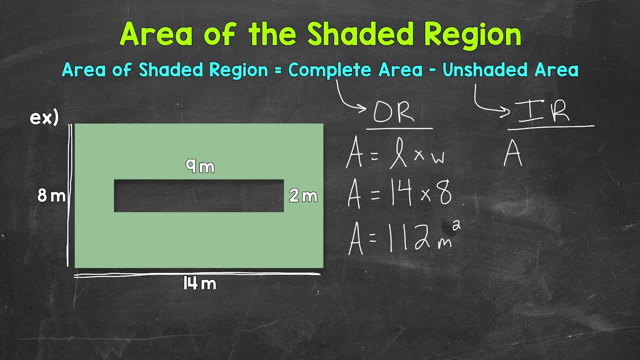 So the unshaded area Area equals length times width. Now we can identify and plug in the length and the width, So area equals. I'm going to use 9 for the length and 2 for the width, So 9 times 2.. 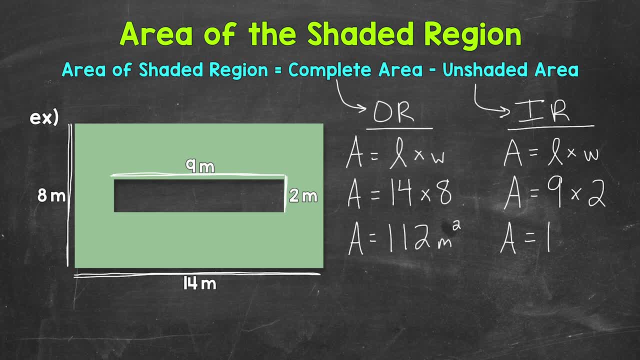 9 times 2 gives us an area of 18 square meters. Now we need to find the area of the larger outside rectangle. Now we have all of the information we need to find the area of the shaded region. So area of the shaded region equals.